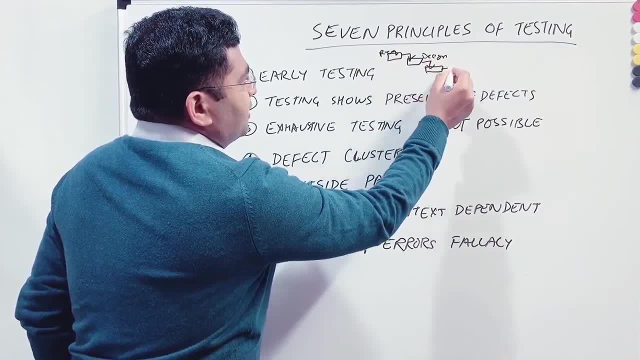 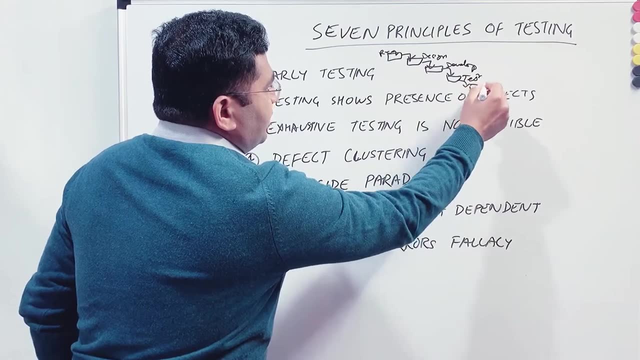 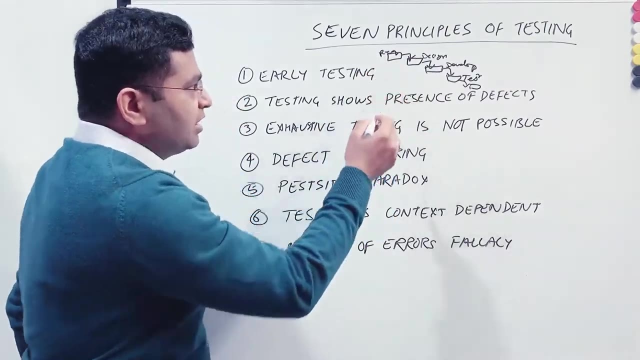 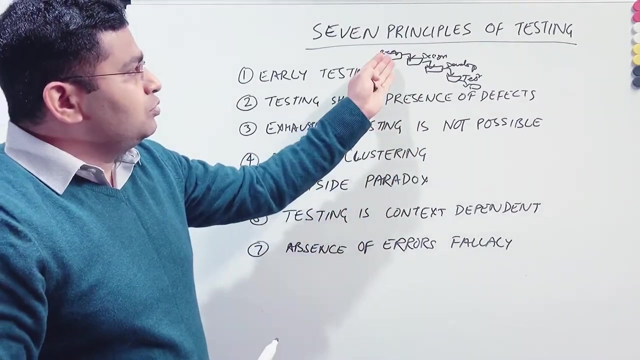 phase. then you have design, then develop and then test and then other you know like deploy and maintenance phase, right, So it was more of a you know waterfall sort of structure and that that is why it was known as waterfall approach. In this particular approach the problem was, you know, you, you had the requirements frozen. 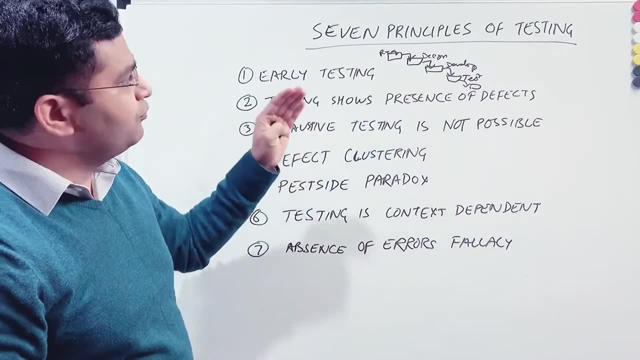 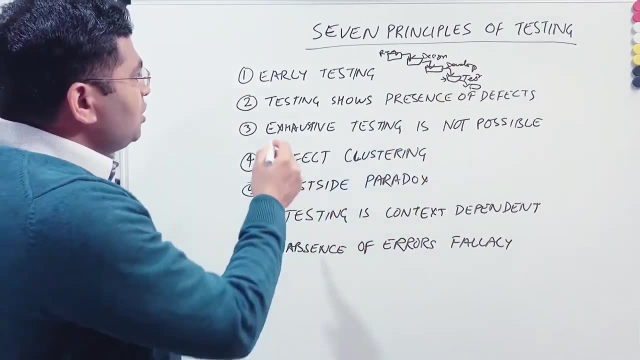 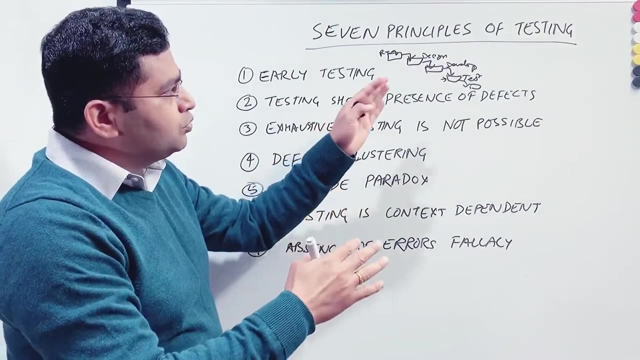 and then you start with the next phase. So a phase need to be completed before you can start in the next phase and you can see the testing came after the development right. So what this early testing principle suggests is: you do not wait for testing in the lifecycle to basically come to that particular phase, You actually start. 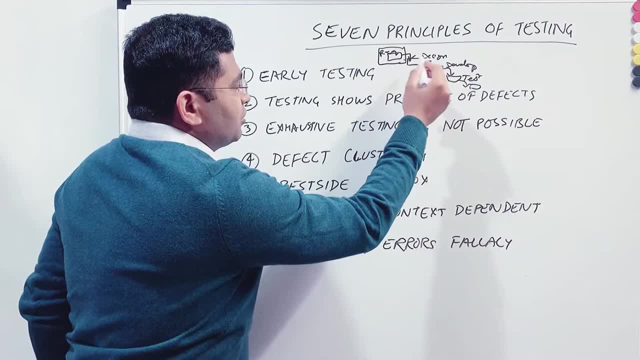 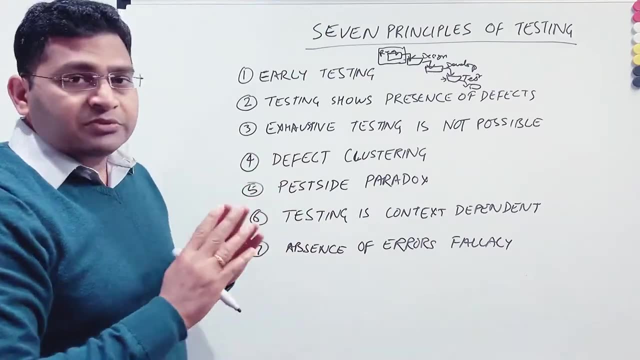 you testing right from at this particular phase or requirement or design or develop phase, In every phase of the software development lifecycle you perform the testing and that's what early testing really is. So if you always that problem that happens like the software development fail, You evolve in the 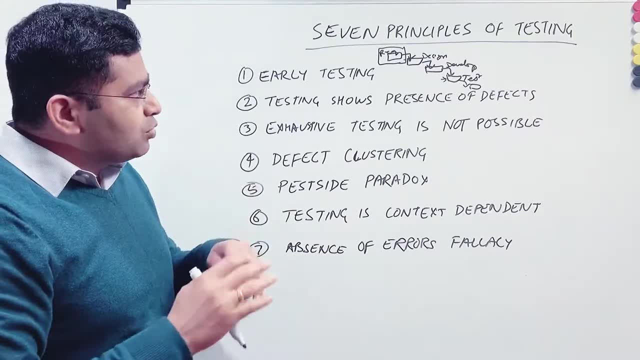 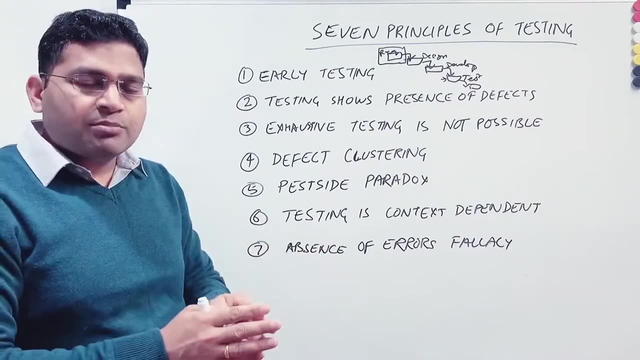 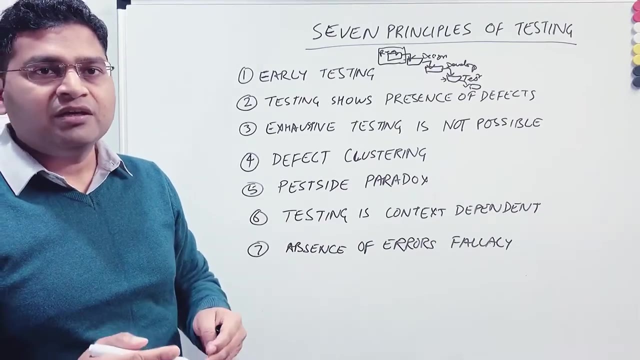 early testing means. Now you would be having a question: how can we test when we don't have anything to you know, like there is no code being developed. So testing is not just about verifying the working code or the working software. It's basically verifying the overall 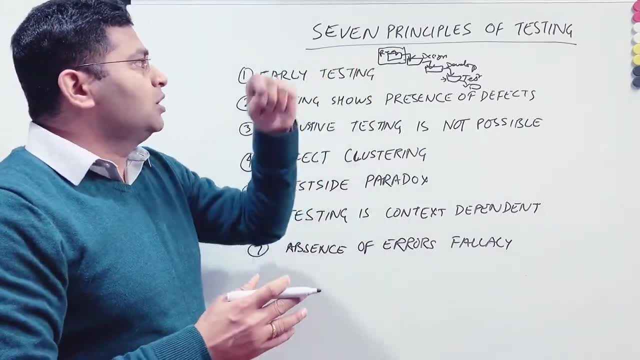 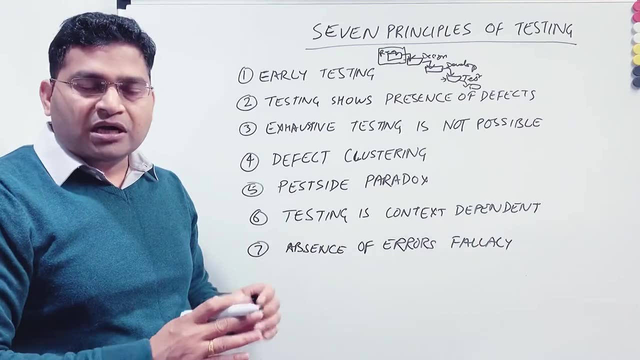 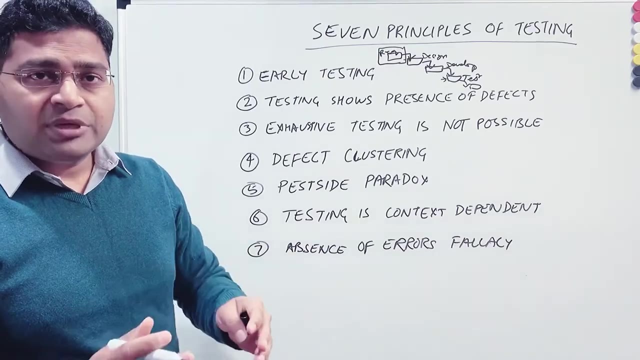 documentation that is being provided. So, for example, you go through the requirement, you get into those discussions with the team and understand what requirements are and how they are being, you know, written, or if there are any gaps that you can determine based on. 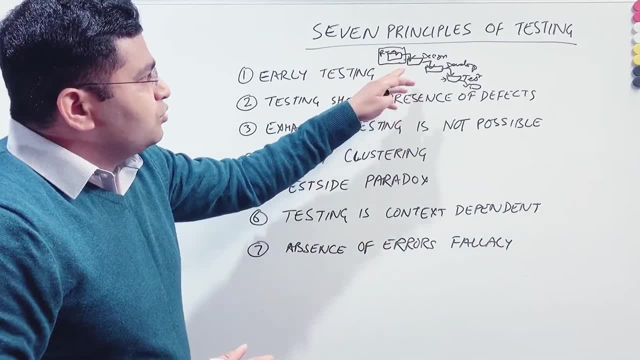 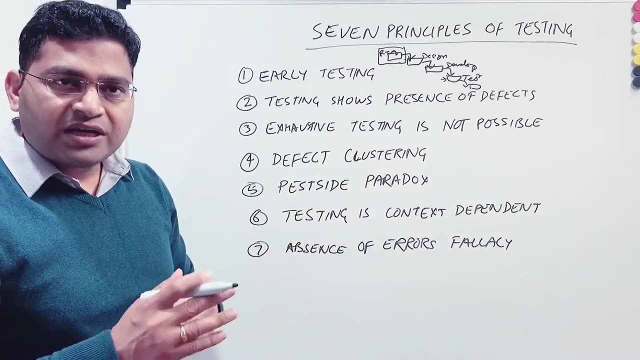 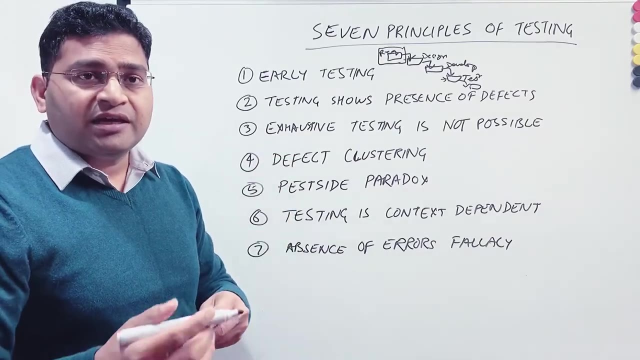 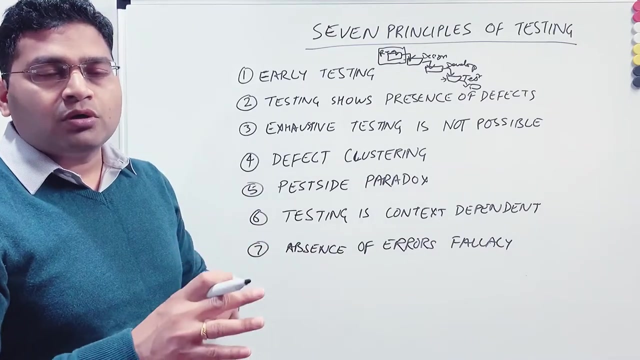 those requirements. Similarly, when there is a design phase, you can go through the design as a tester and understand how the design is defined or how the overall design is and how you are going to basically test it and put the tester's you know hat and understand, based on the design, how the overall 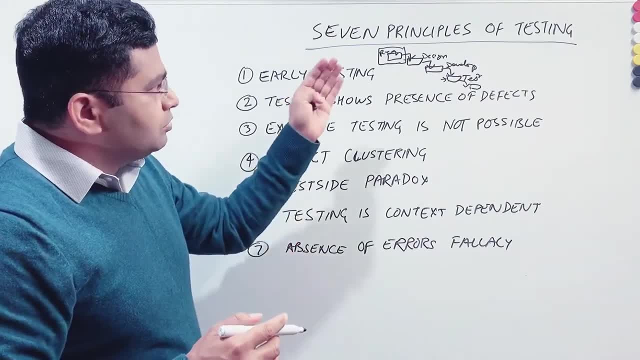 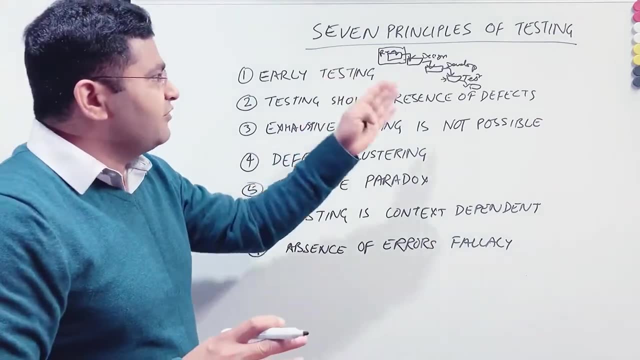 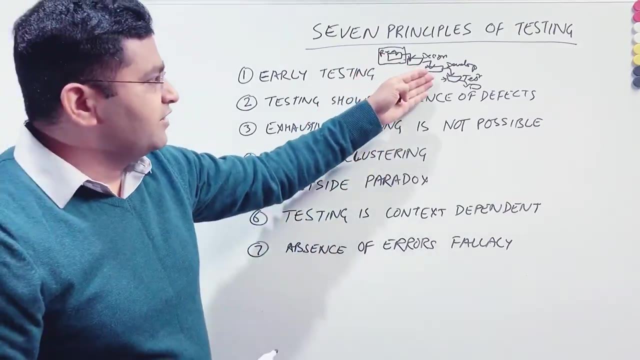 software is going to function. So early testing says that you do not wait for testing until the testing phase is there in the development lifecycle. So that's the first principle. Now, this was the problem with the waterfall approach: that testing phase was coming after the development phase, or 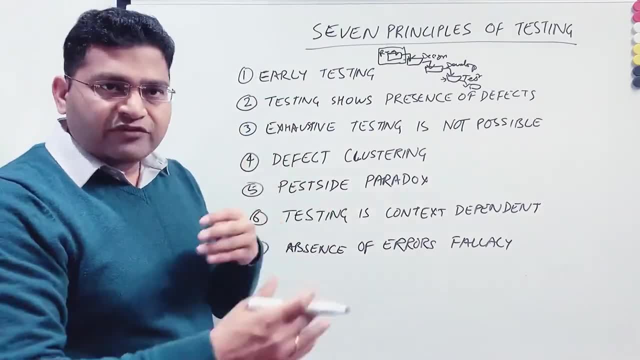 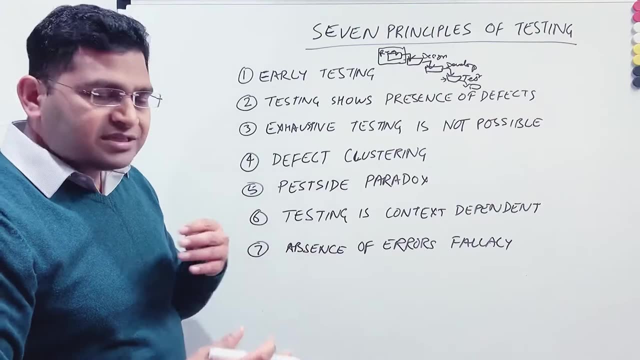 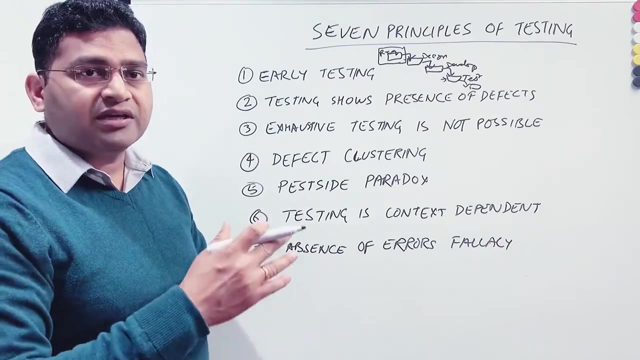 multiple phases When they got completed, And that is why the development approaches have evolved, and agile or scrum is the latest one wherein you know you have shorter iterations. so you test almost in every cycle. I mean you test in every cycle, not almost, it's every cycle or every iteration you test. 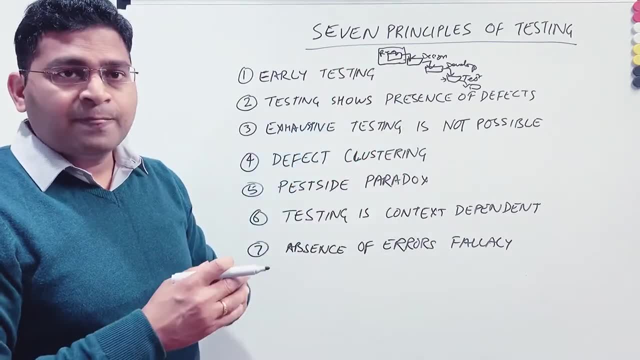 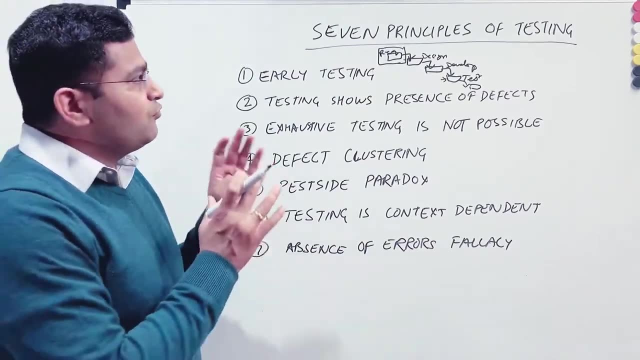 And you test in all the phases, Right. So phases, I mean there will be requirement, there will be, you know, design in a smaller, shorter iteration as well. But testing is in involved in all the phases of software development life cycle, and that is what early testing is all. 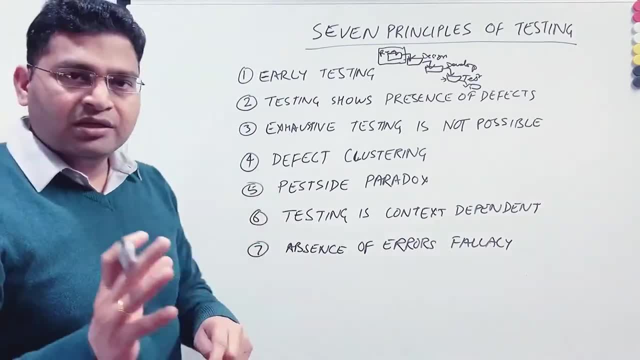 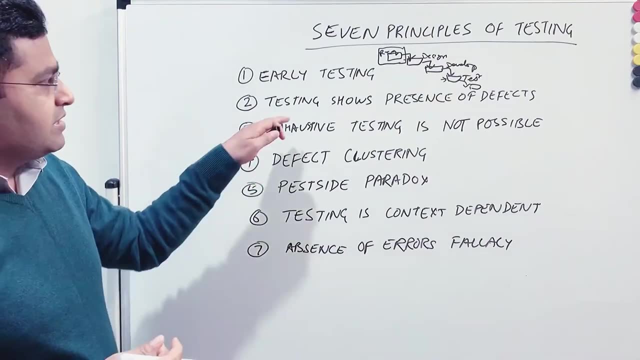 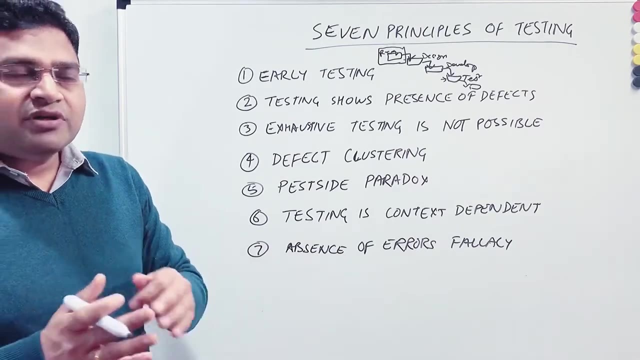 about you start testing as early as possible, right? so that's the first principle. the second one is about testing shows presence of defects. now, testing will show that the defects are present in the software, but it can never show that the product is defect-free. we have already understood. 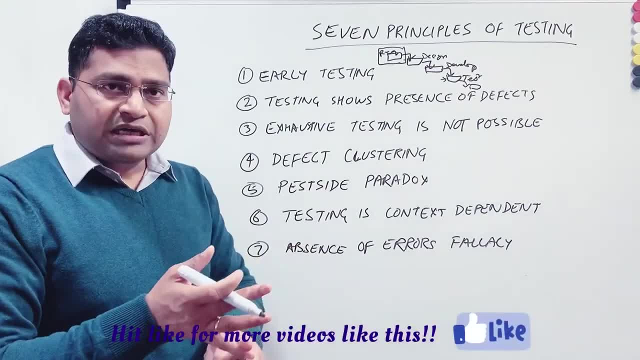 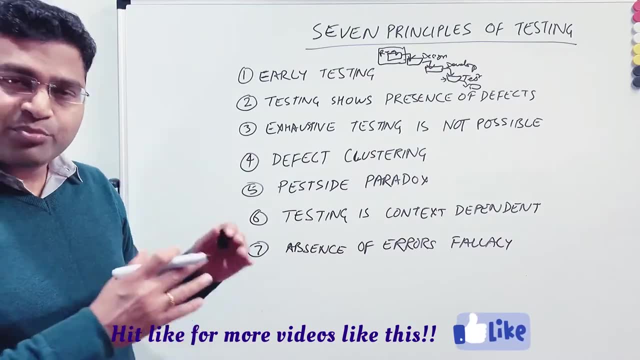 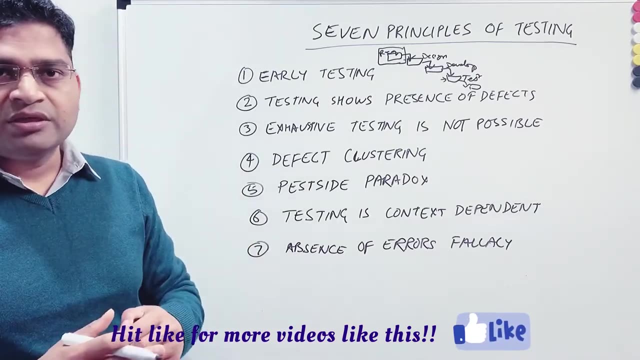 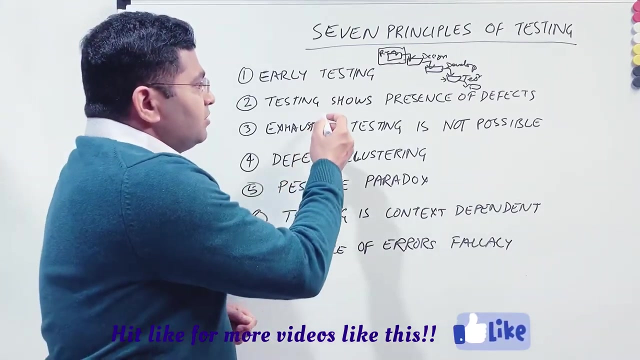 about the examples of big organizations. uh, you know, yahoo, flipkart, where they have? you know, even though they had such a huge testing capability, still their product or the, the softwares that they launched, had failed in, you know, in different circumstances. so when these organizations would have tested those software, they would have tested it thoroughly. 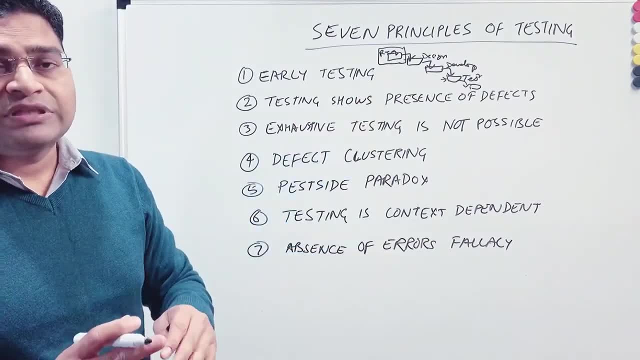 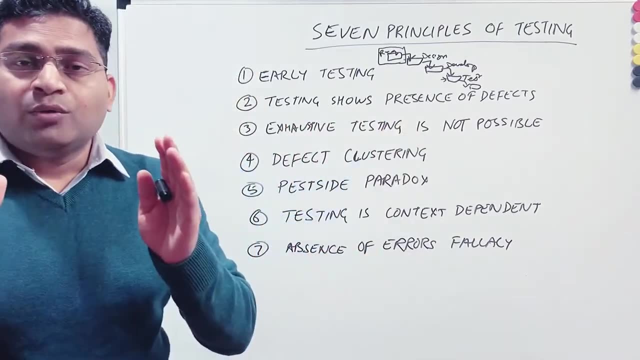 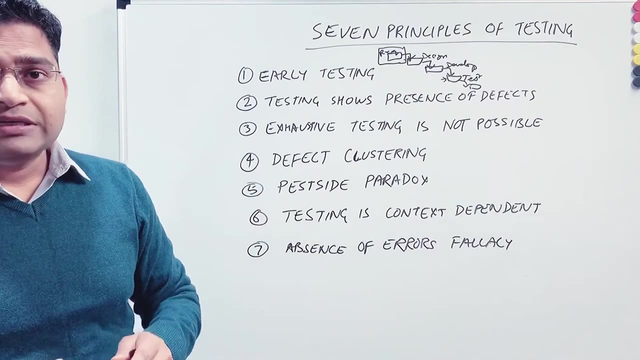 so testing shows the presence of different, but it never shows that the product or the software is defect-free, right? so that's the second principle and that is why, when the software is deployed into production, you will see the production defect coming through right. so, based on different circumstances, a software, 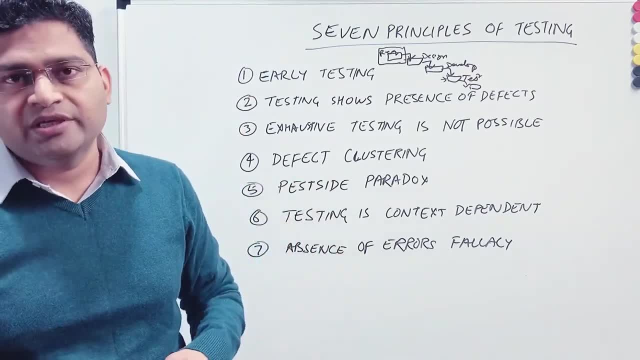 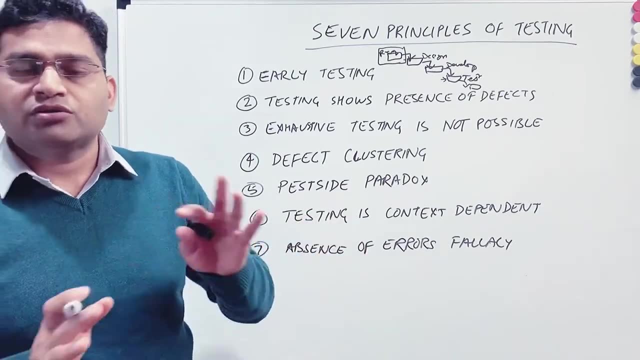 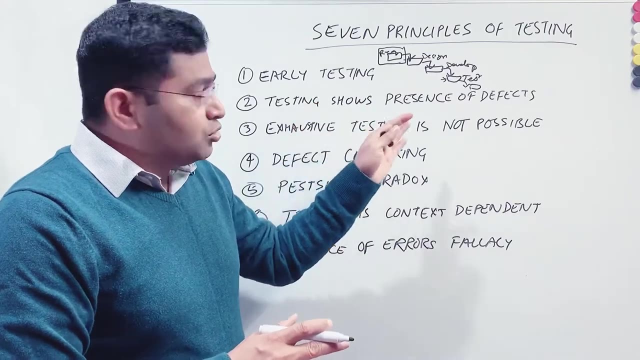 which might be working now in your test environment might not work in you know uh production environment or uh, maybe in production environment. there is some difference in the hardware or the software, right, so that you can't exactly replicate in your software or in your testing environment. so testing shows presence. 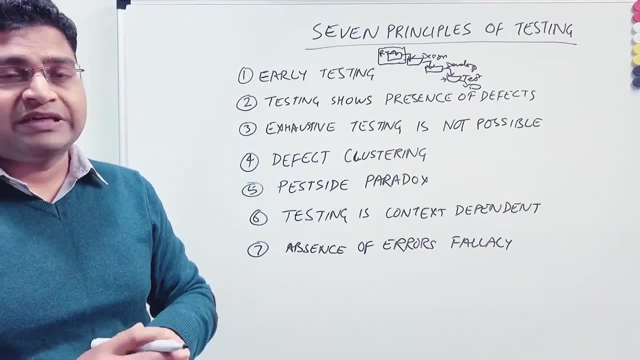 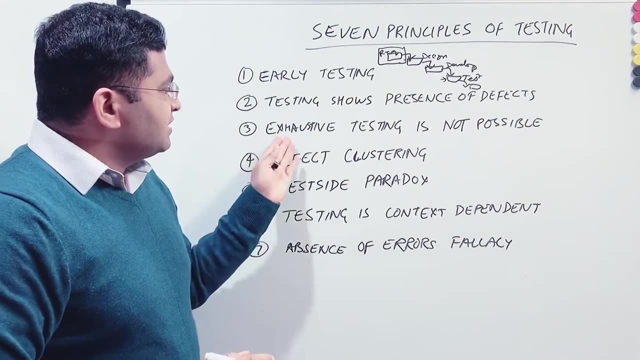 of defect, but it never. you can never claim for a software that my software is 100 percent defect free and it will never fail, right? so that's the second principle. third principle is: exhaustive testing is not possible. what this means is exhaustive, so exhaustive testing is not possible. so 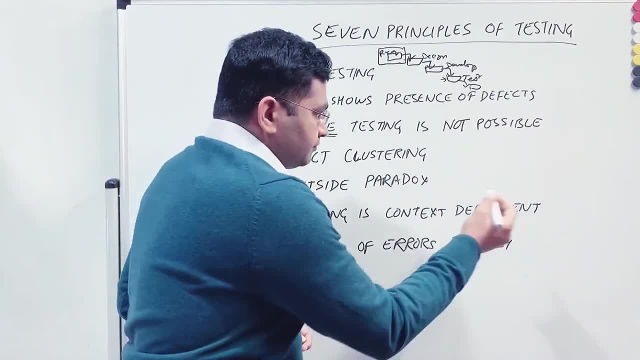 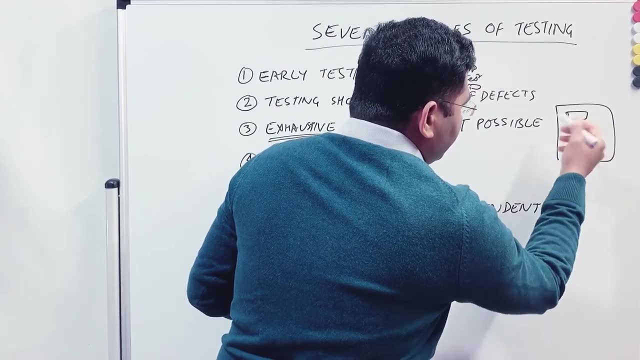 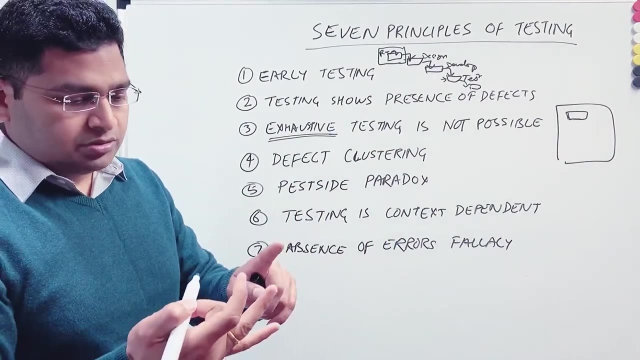 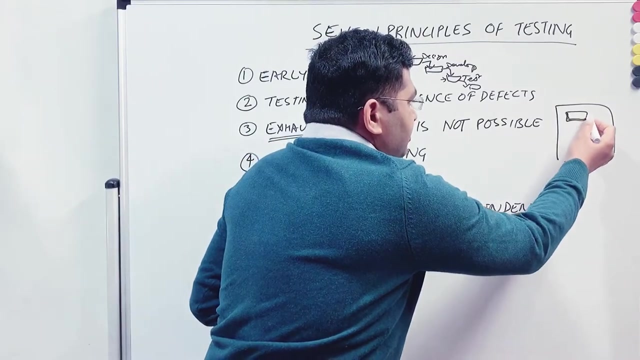 say, for example, you are testing a web page, right, and a web page has, say, for example, you know this particular text field right which just accepts one character in it. okay, so it could be number, you know it. it it accepts any of the alphabet, say, for example, one character. so just to test this hundred percent, this text box, hundred person, because it. 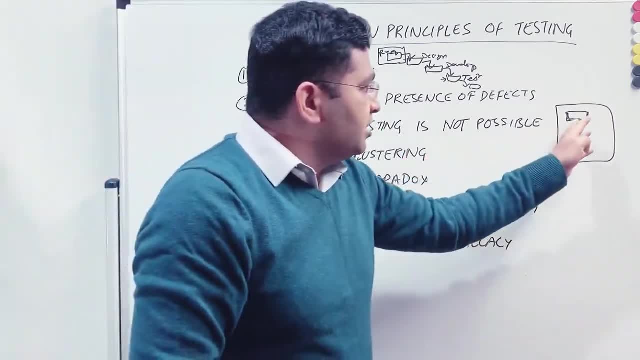 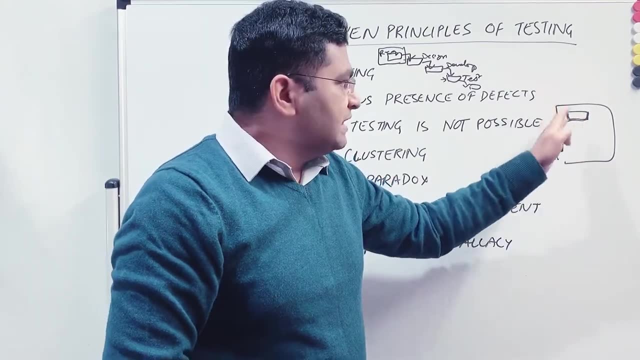 accepts one character at a time, you need 26 compounds, combinations of, you know, uppercase, 26 combination of lowercase, right? So if it just accepts those characters, and then you have to go through the negative scenarios, right? So you have to. 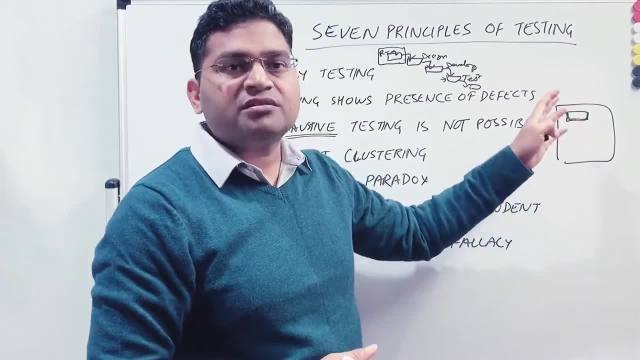 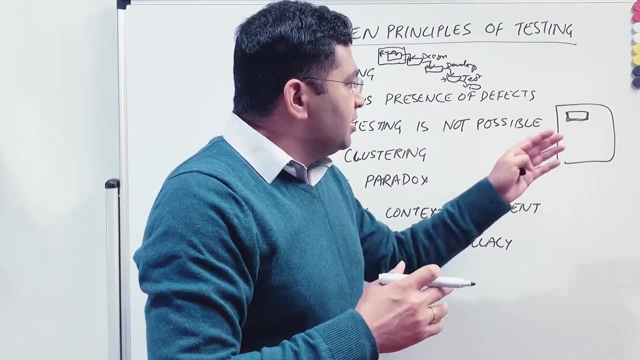 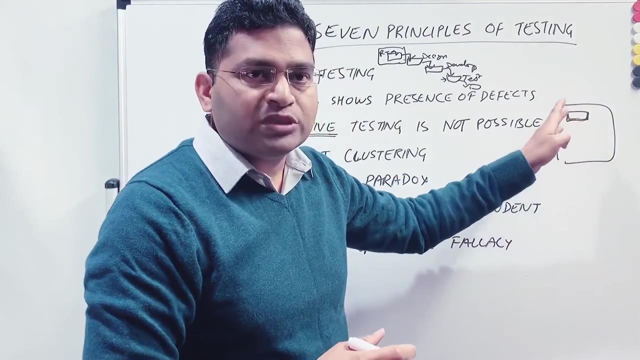 basically go through and test with the special characters that it's not, you know, accepting any of the special characters or any numbers. So you can imagine the amount of combinations that you have to test this particular text box which just accepts one character right Now. say, for example: 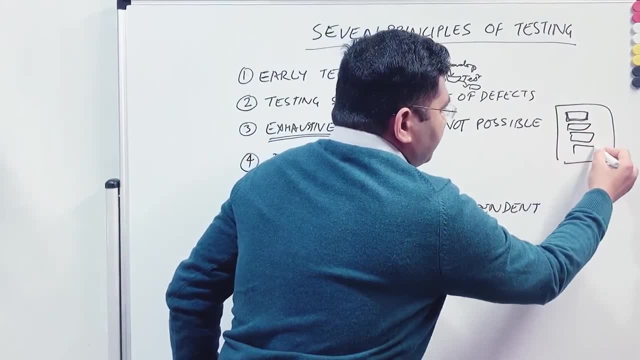 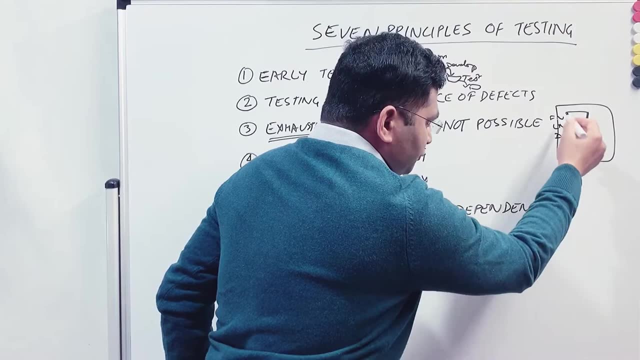 in your web page you have, you know, a couple of text boxes. So first name, last name, right date of birth, So these, you know, are very commonly web page text boxes that are available right. So now. 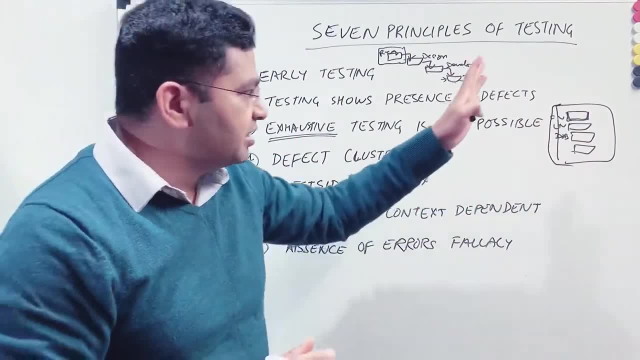 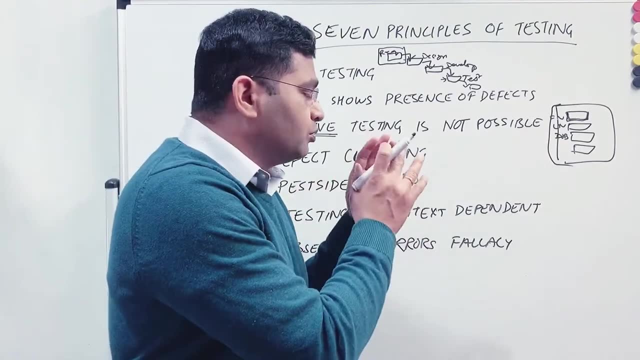 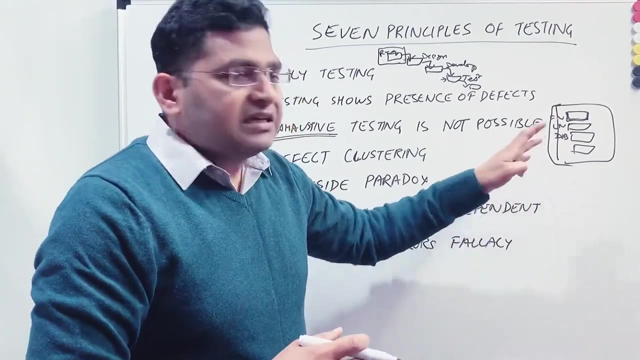 if you have to test all these text boxes that are present on a particular web page with so many different combinations, it is nightmare. even though, if you are using the automation tool to do all those permutation combination, it is not possible, right? It is highly unlikely that you will be able to. you know. 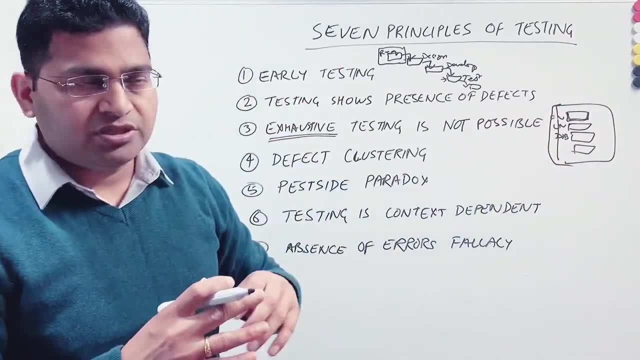 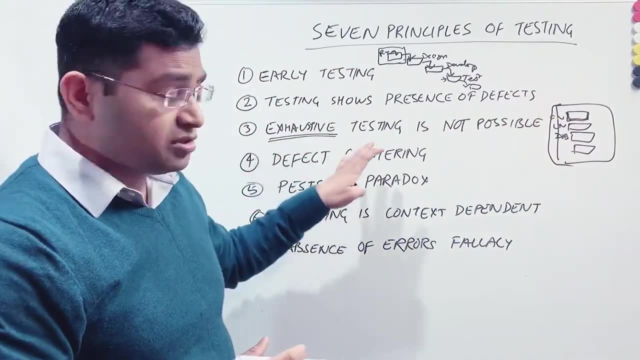 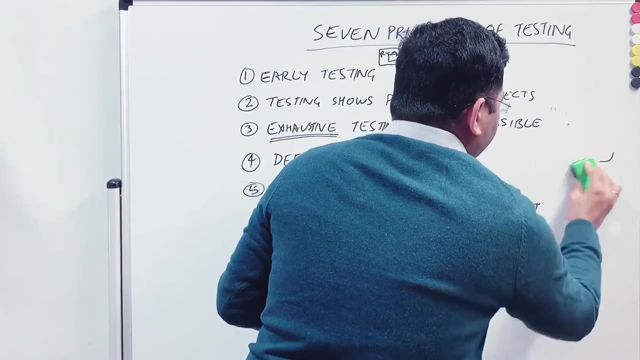 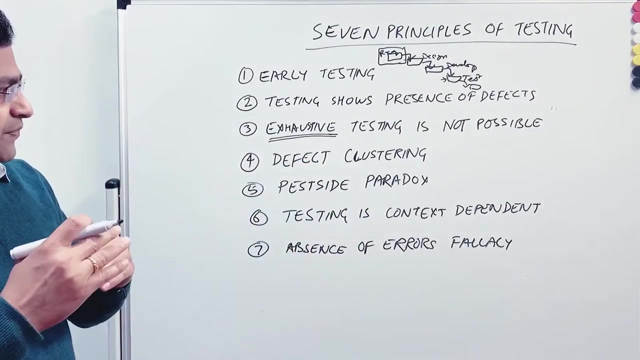 achieve 100% of the combination or the possibility of exhaustive testing for any of the software applications. So, third principle: exhaustive testing is not possible. okay, The fourth one is defect clustering. right. So what this means is that defects are found. So most of the time, 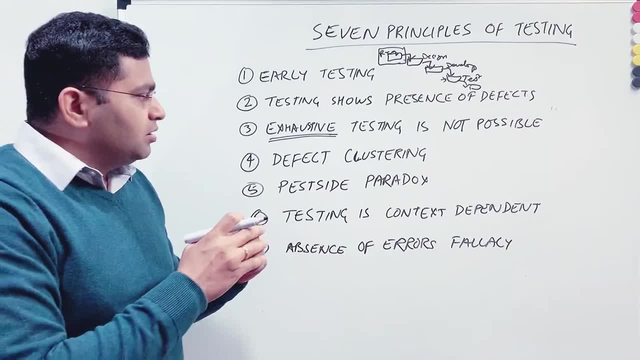 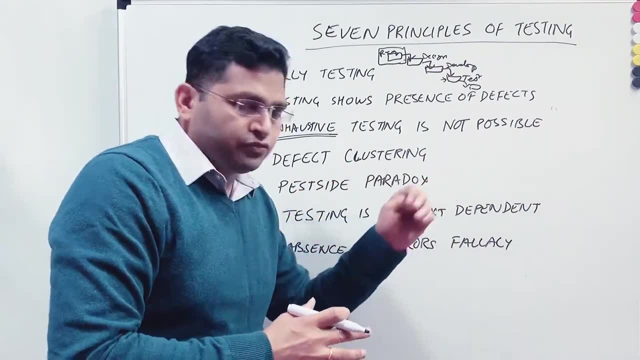 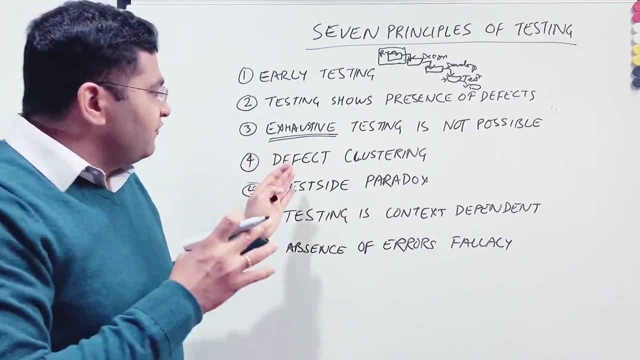 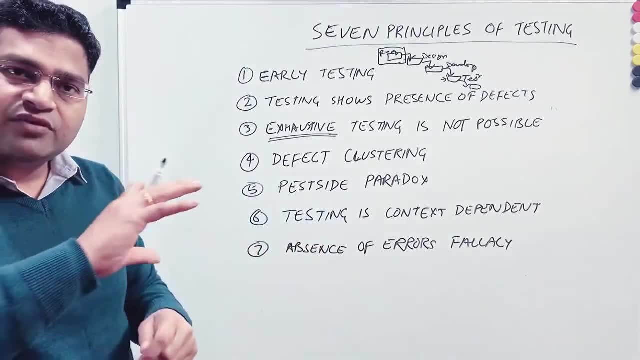 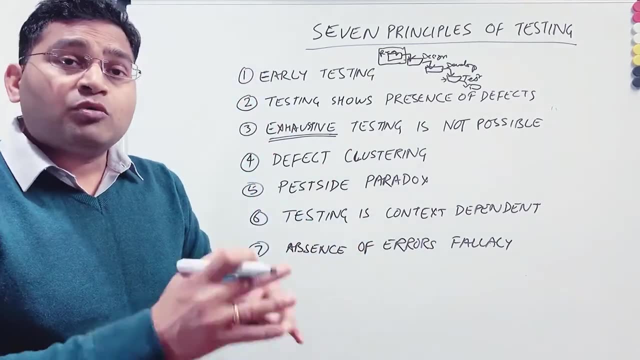 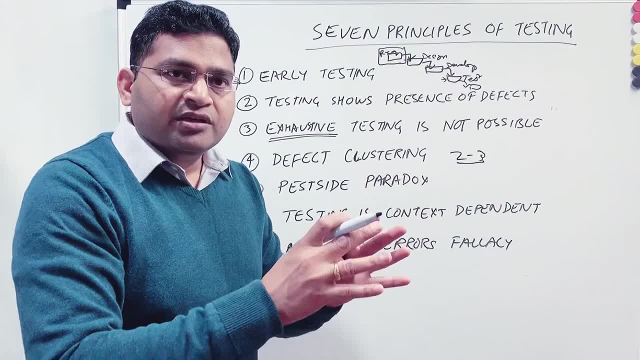 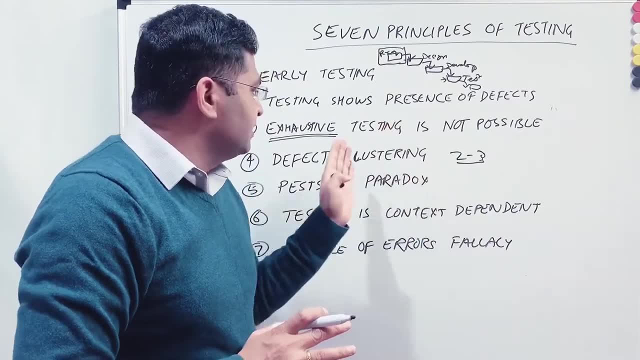 right. So wherever you will find a lot of defects and those defects are related to particular modules, most of the chance, or it's highly possible that those modules will have a lot more defects, and that's what defect clustering is, Defects are. 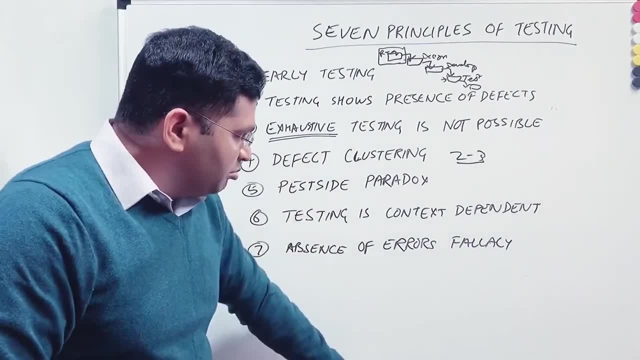 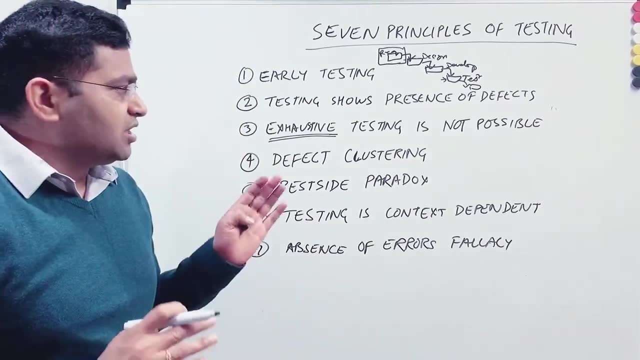 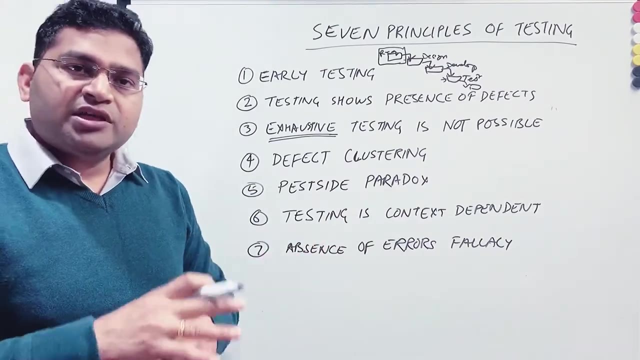 clustered in few particular modules of the software because of the complexity of those modules, the integration etc. So it might be possible that defects are clustered for those particular modules. and simple modules are the modules where you don't find much defect. there won't be a lot. 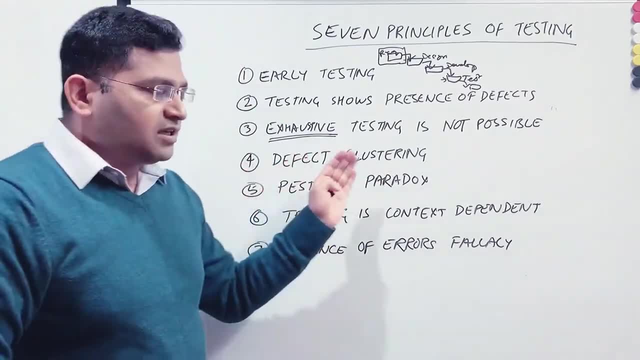 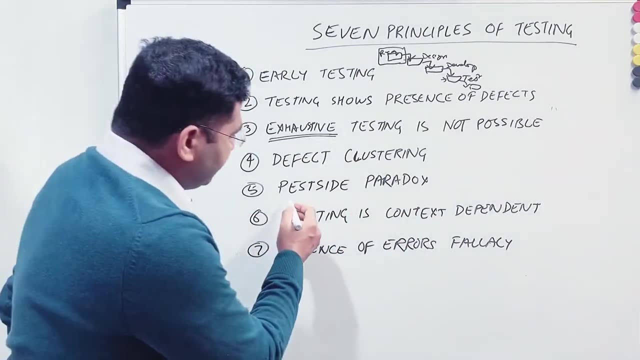 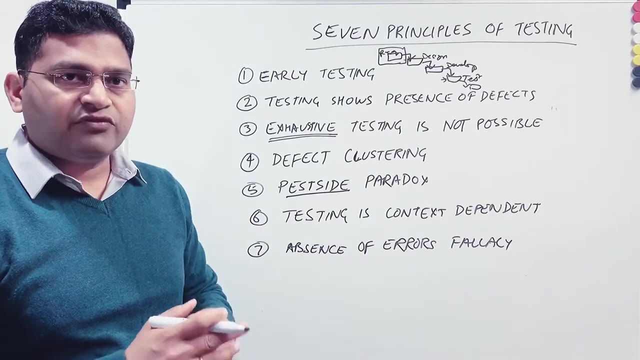 many defects in this. So that's the fourth principle of testing: defect clustering. all right, Then you have pesticide paradox. Now, as the name here pesticide, so pesticide, as you see, even in agricultural, you know, agriculture or farming. when you use same pesticide again and again in the crop. so at some particular time that pesticide stops working right. So the the pests build the immunity against those pesticide. So same pesticide is not going to work for those pests anymore And similar is. 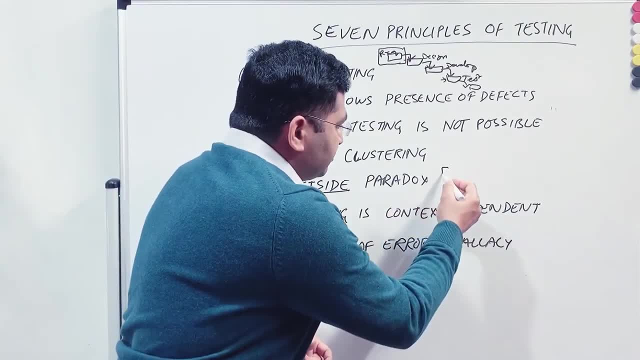 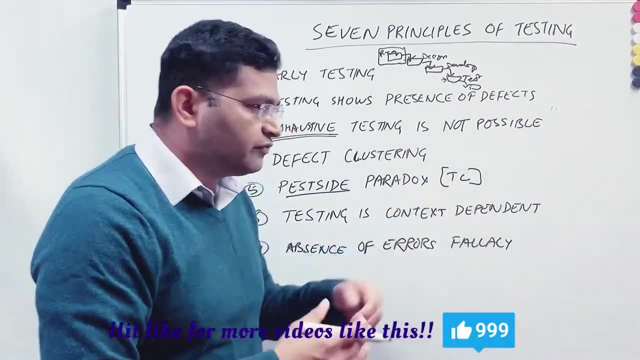 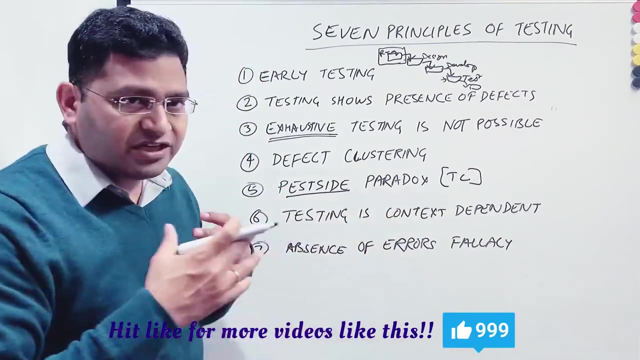 the case in the testing. So if you are having test cases and same set of test cases, you are executing for each and every version of the software again and again to try to find out new defects. it's not going to help you out. In order to find new defect, you need to have the new set of test cases, right? 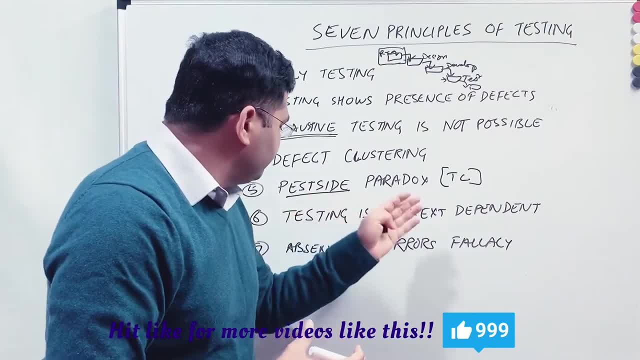 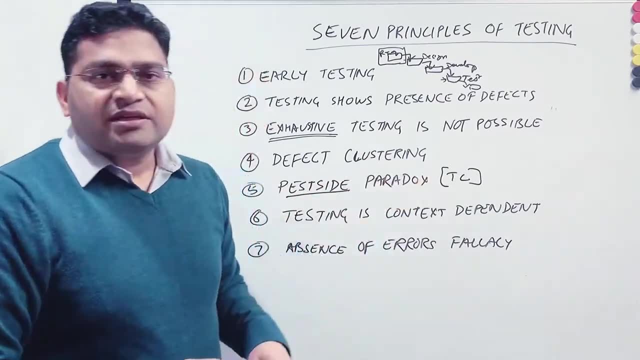 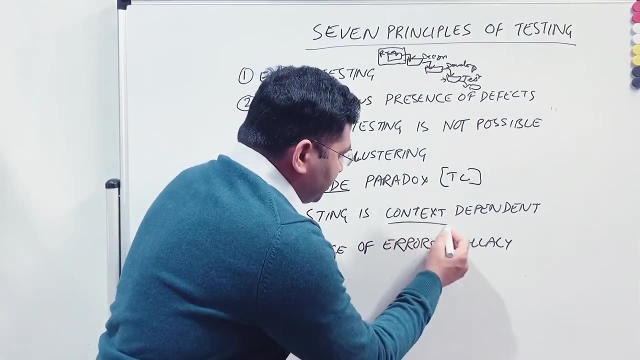 Same test cases won't find you new defects. So that's the fifth principle: pesticide paradox, similar to what pesticide does for the crops. It is same with the testing. all right, Then testing is context dependent. What does this context mean? Now say, for example: 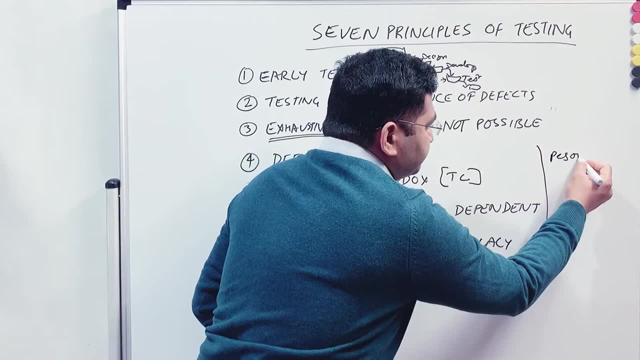 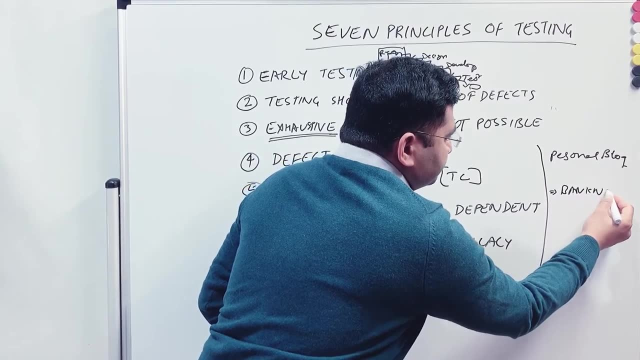 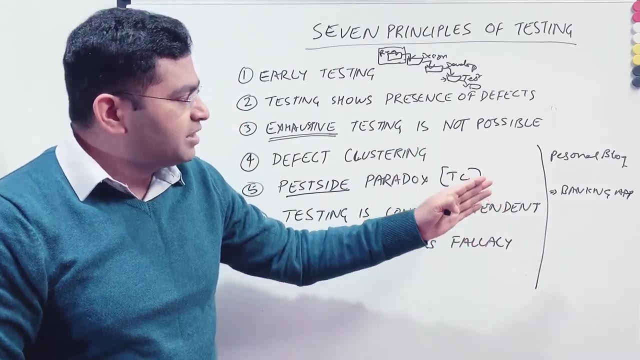 I'm testing my personal blog, all right, And then I'm testing a banking app- okay, So banking app will basically, or how you are going to test banking app. the context or the complexity will be completely different for the banking app as compared to. 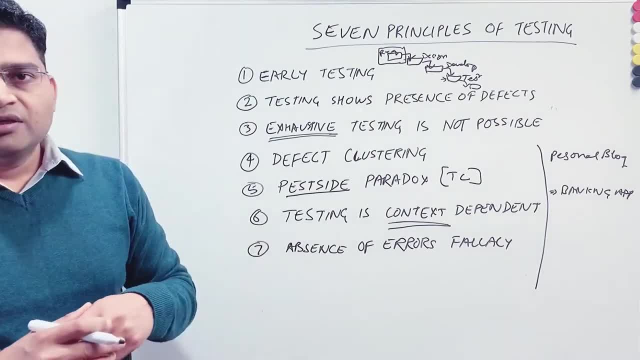 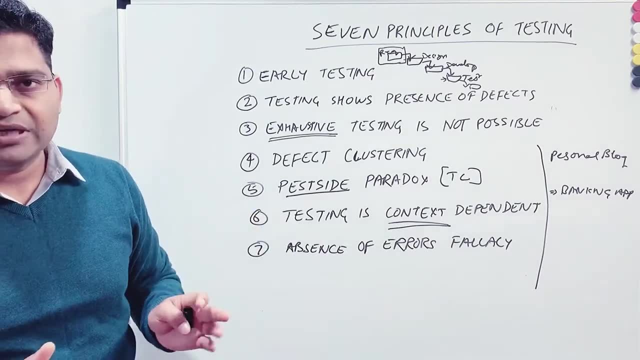 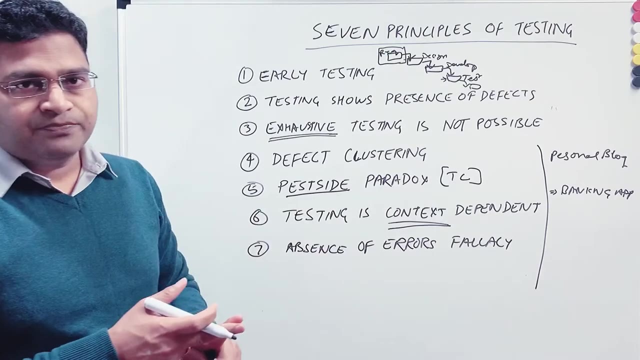 personal blog, because personal blog is very minimal set of features and even if there is, you know some features that are not working, it doesn't impact much, right? i mean, there is not a lot of you know revenue impact or there is not a no you know um other any other sort of impact. but in terms of 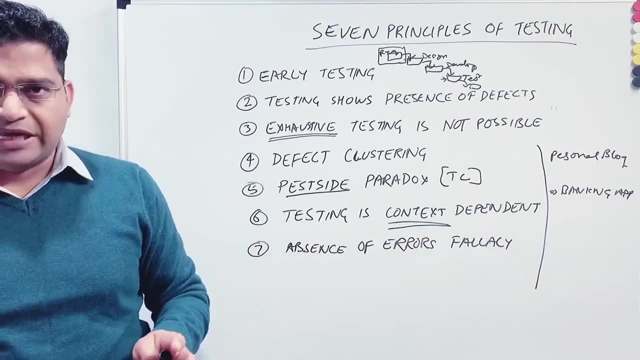 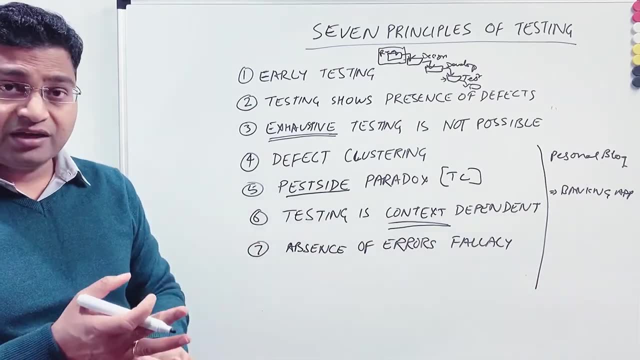 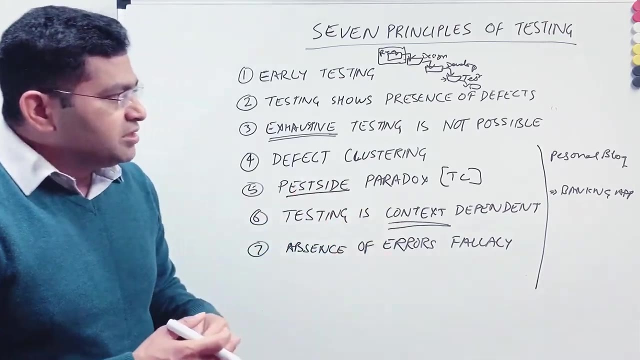 banking app. there are so many customers for a bank that rely on the application, so if that application is down i might, as a bank, lose the reputation and lose the customers. so revenue okay. so testing is context dependent. means it depending which sector or which you know field you are? 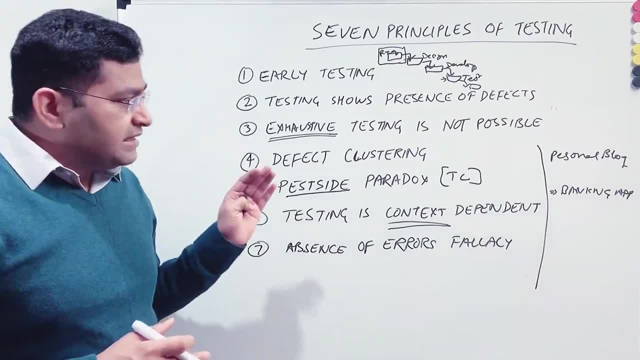 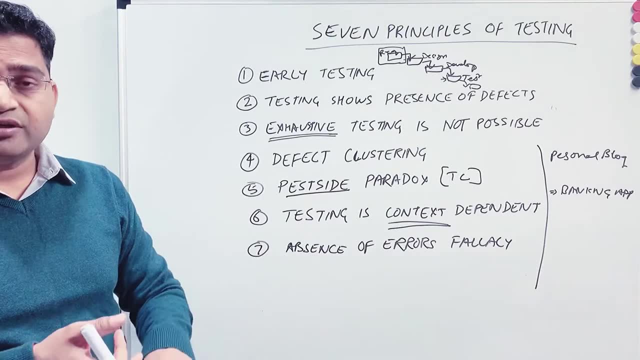 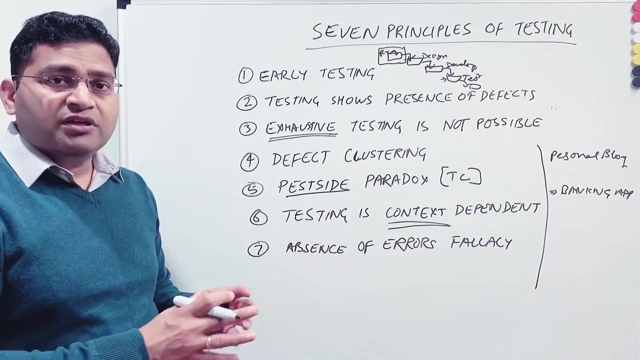 trying to test or which type of software you're trying to test. test type will depend based on that. so banking app um will have more rigorous, you know, testing if it is safety critical or you know, like airplane uh software. there will be a lot of other criterias that you need to fulfill in order to 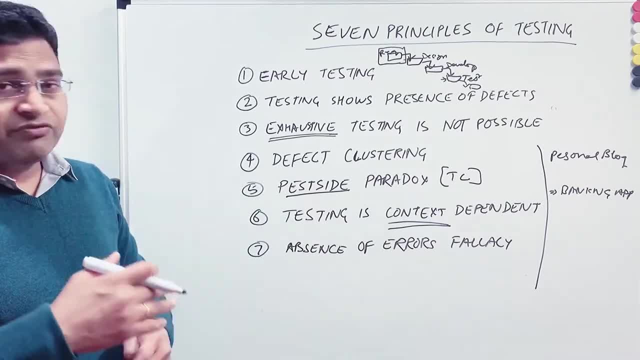 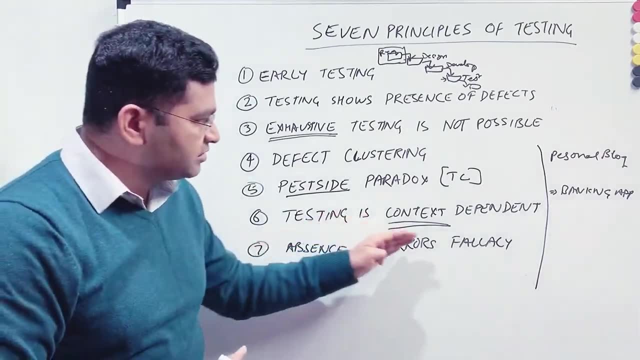 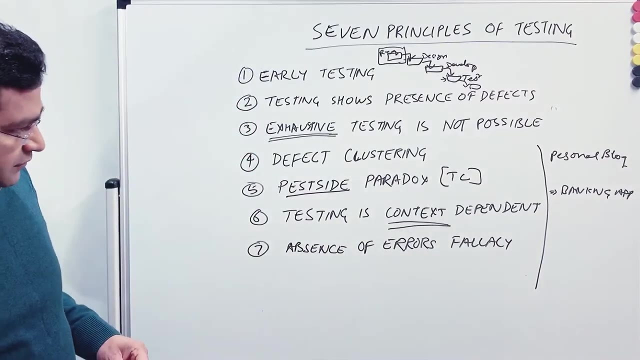 say: yes, this software is tested successfully, right? so even documentation that needs to be generated for different, you know, context will be different, right? so testing is context dependent. is sixth principle of testing. then absence of errors, fallacy. okay, so what this means is say, for example: um, i have a software and i have tested, you know, that particular. 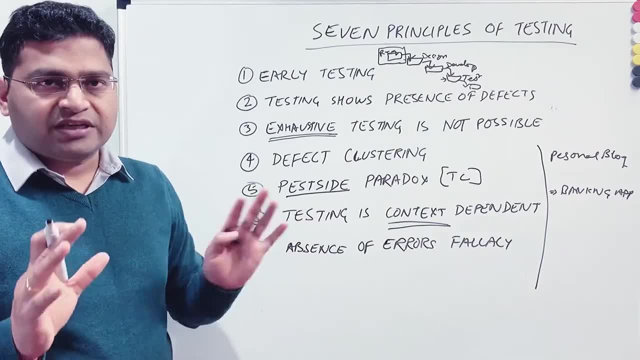 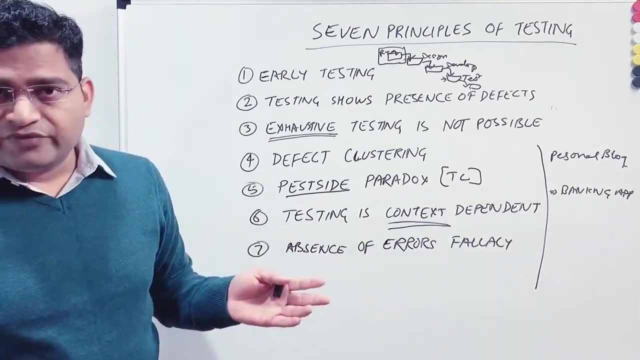 application and that application doesn't have any defect as such. i mean, i've tested it thoroughly um all the test cases that we have written have passed and there are no defects, outstanding defects. we have fixed everything, all right now. similar example i'll take, you know, um customer. 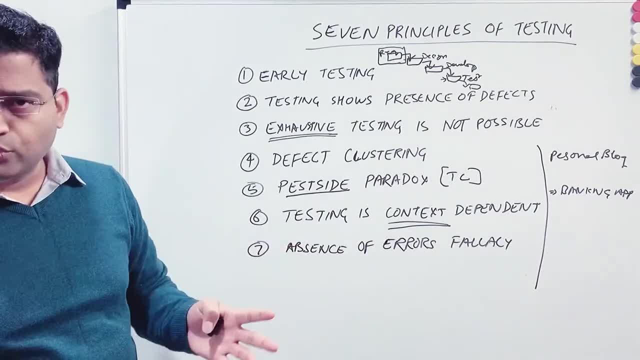 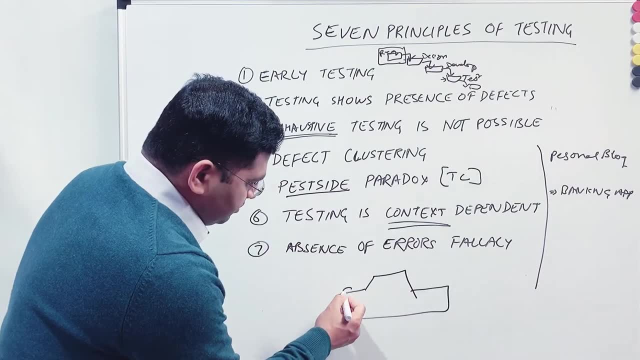 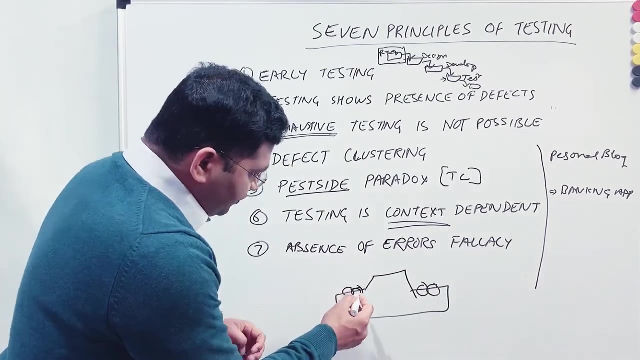 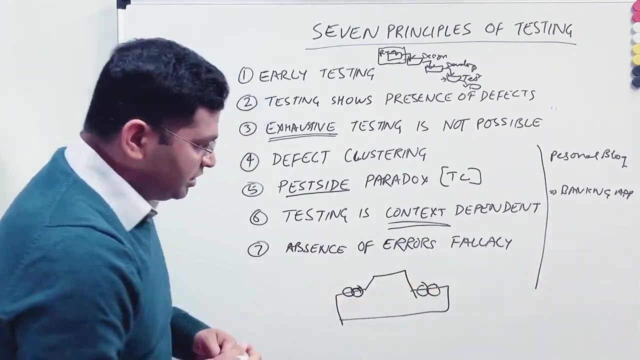 gave us a requirement: i need a car with four wheels, okay. so, um, you have this car and you have put four wheels, okay, so it meets the requirement and four wheels are there. so when you will try to, you know, test that. yes, for are there four wheels in a car? yes, there are four wheels in the car. 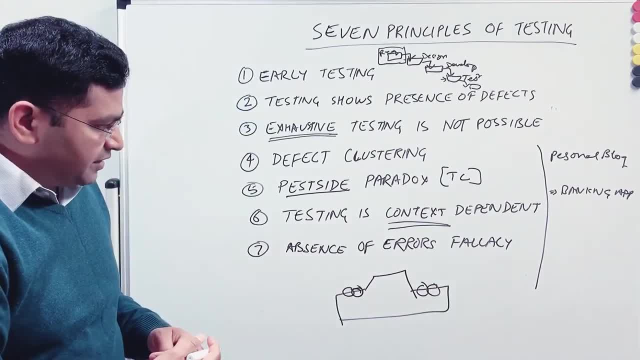 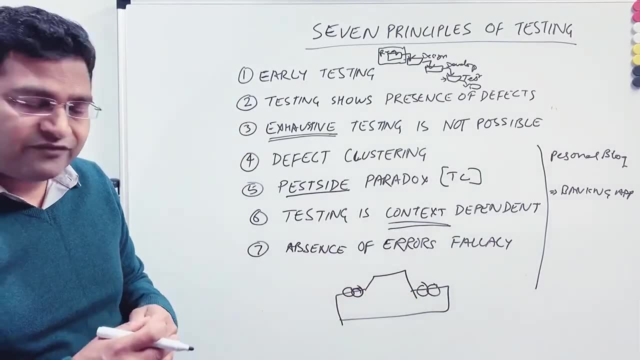 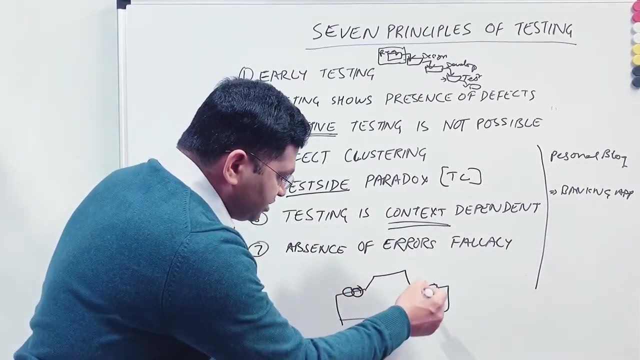 um, and this is, you know, like a car shape. but then you did clarify that where these wheels are, you know a exchange and so you've used the 400 wheel show it. so you did clarify that where these four wheels right is what the four wheel should be right. so there is, there is nothing. 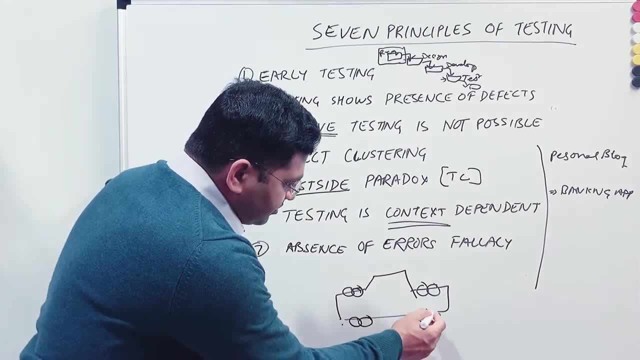 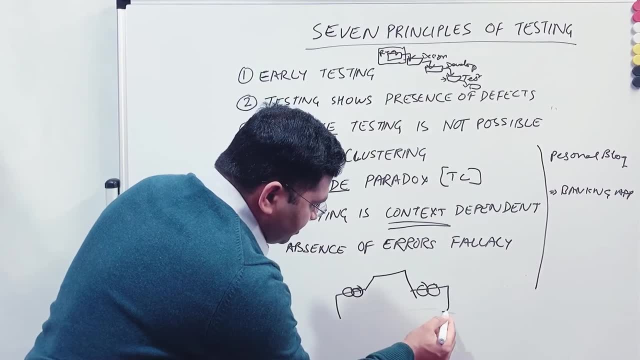 that you've clarified whether this car will be fit for use or whether this is what the customer wants. the customer wants wheels at this particular location, or he wants wheels at this particular location so that car can move right. so you didn't clarify that from the customer. 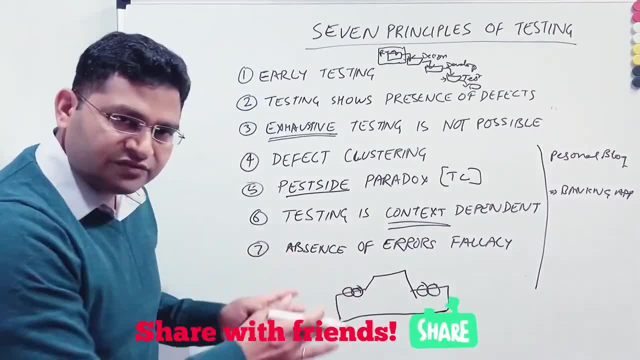 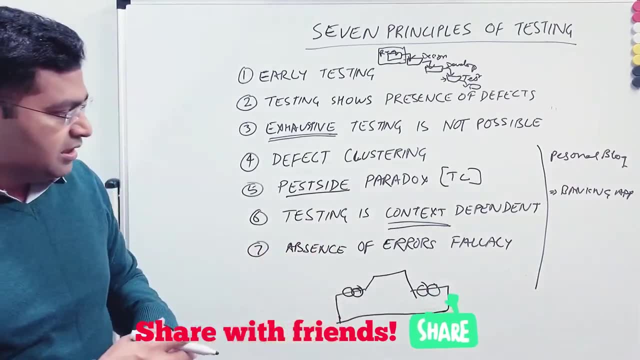 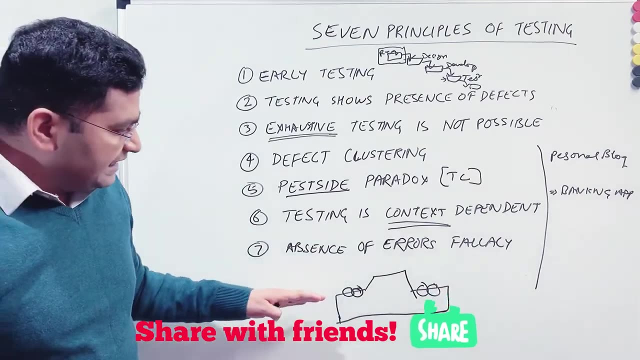 and based on what requirements customer has given. you have verified and you have said: yes, my software or car is defect free, because customer told i need a car with four wheels and i have put four wheels. four wheels are there and this should be fine, right? so this is not fit for use and this is. 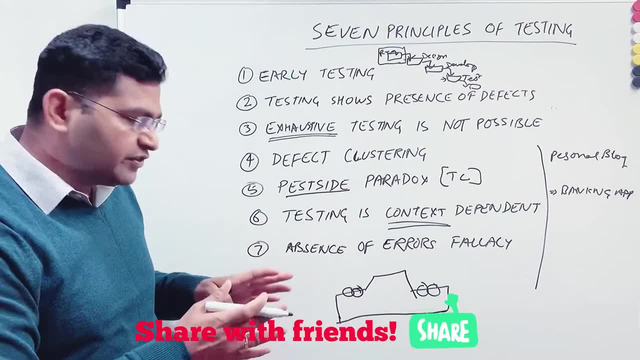 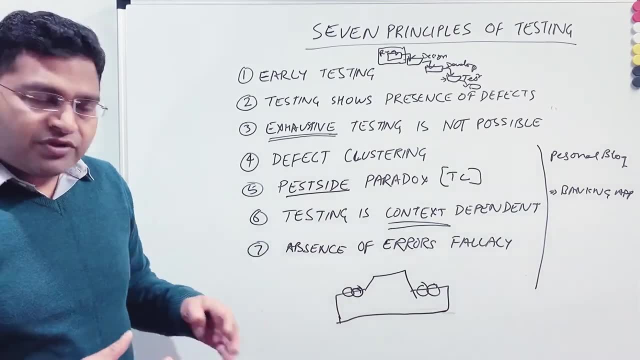 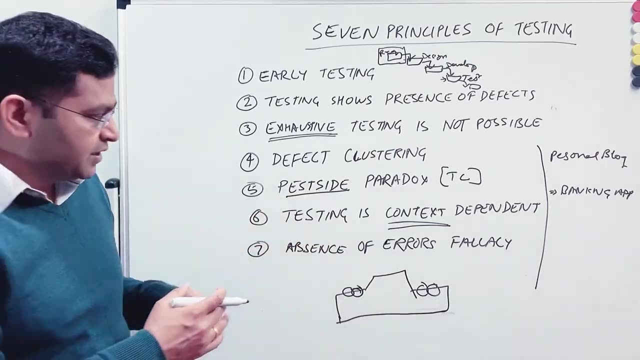 what absence of error policy is so if they, even though, if there are no errors, right, even though there are four wheels and all four wheels are rotating properly, even though this you know there is in terms of what requirement customer has given you, meet those requirements. but if it is. 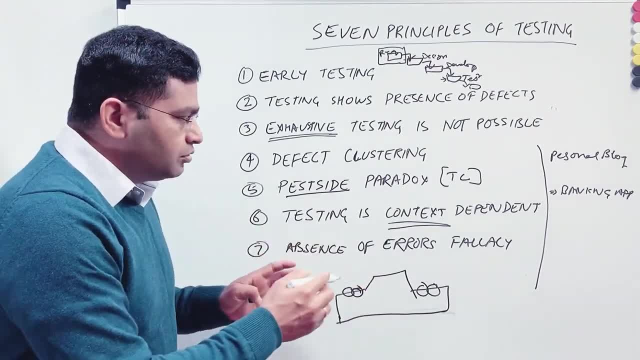 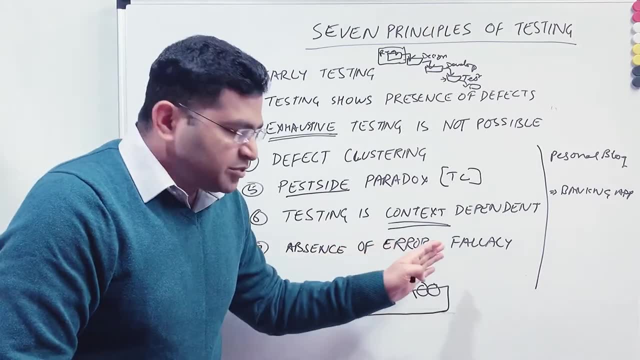 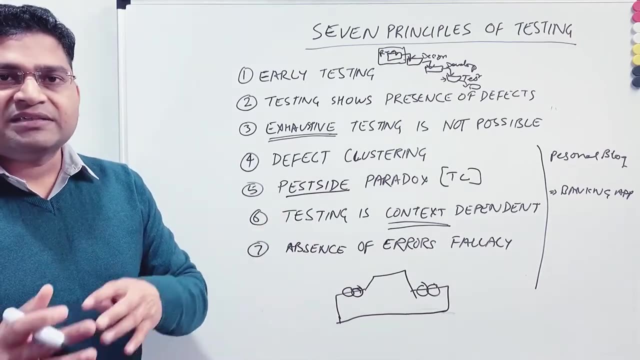 not fit for use, then that is not good, even though there are no errors or no defects in the software. okay, so this is absence of error policy. basically, if your software doesn't have any errors or bugs, that doesn't mean that it is still fit for use, unless and until you question your customer. 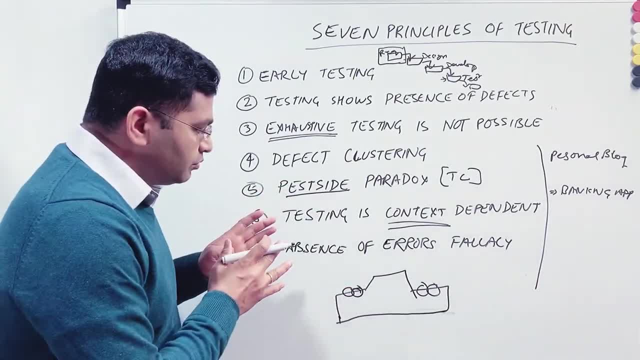 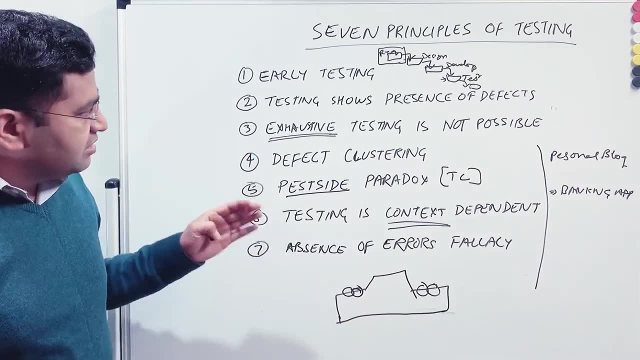 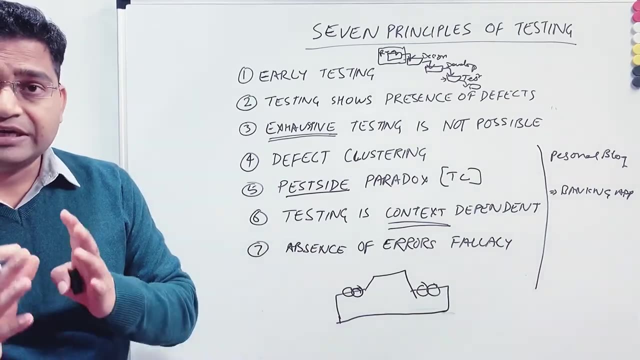 or you, your client, that you know whatever you have developed is what he needs or is fit for use. all right, so these are seven principles of testing. i hope these were helpful and clear for you to basically understand and if you go into any interview and have been asked any of these, 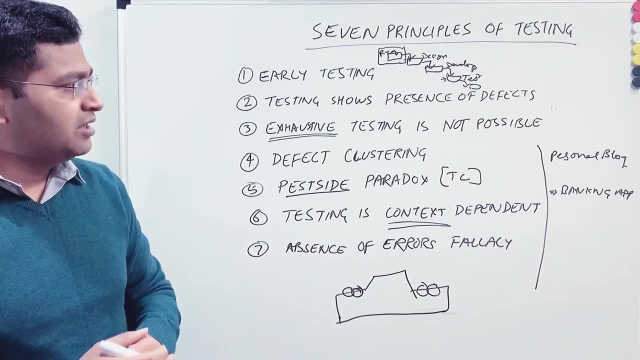 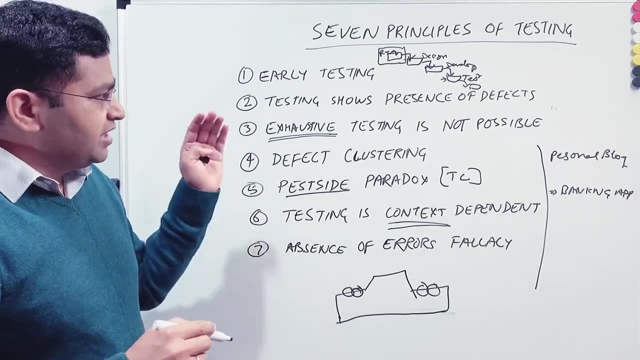 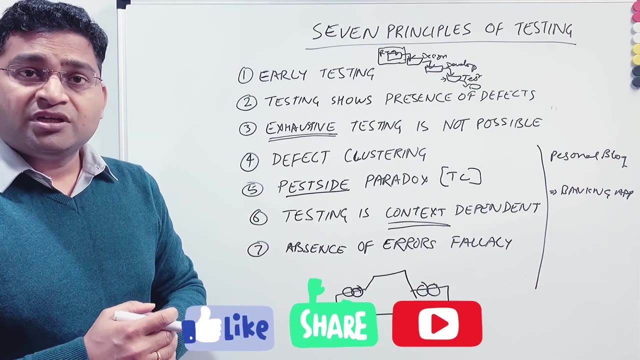 you know principles, you would be able to answer them very clearly. if not, please comment out in the comment section below and i'll try to clarify any of the doubts that you will have in any of the principles that we have explained here. all right, so that's all for this tutorial. please do share. and subscribe and thank you for watching.